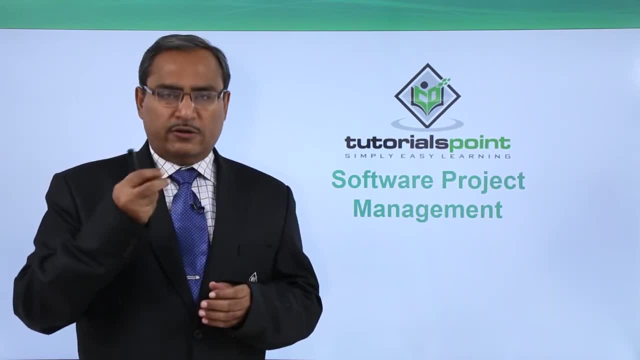 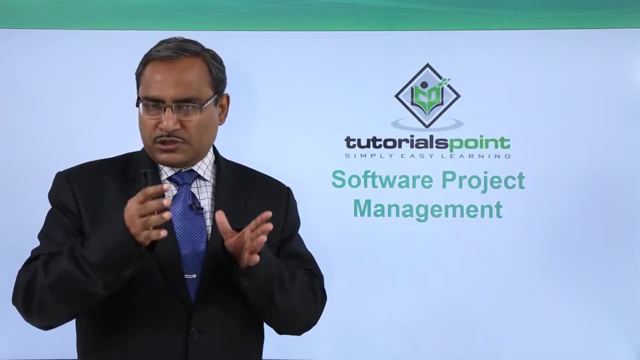 of that, we are going to get one new result. There is a new innovation, So that should be considered. That means doing the doctorate, going through this doctorate program study. obviously, that is nothing but a project, Because at the end we are going to get unique result Whenever we 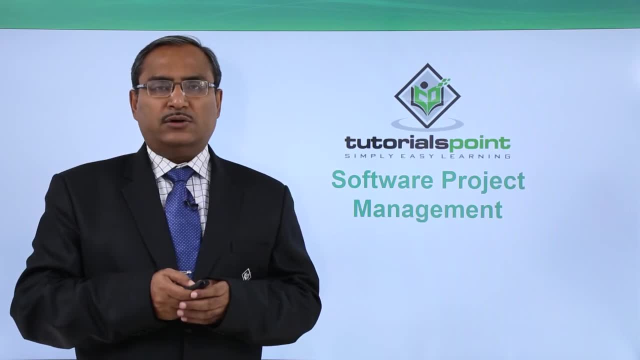 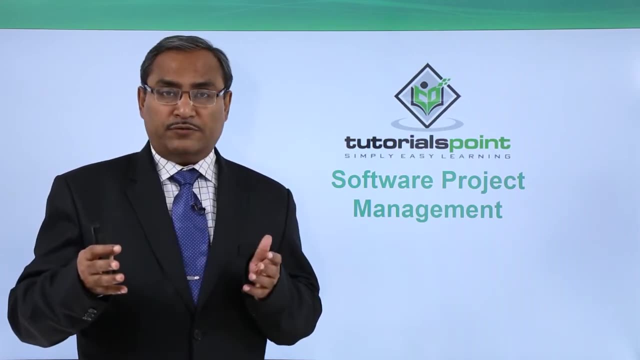 develop software, then obviously each and every project must be having a specific start date. So each and every software has got different recommend list, different client, The different might be. the platforms are distinct from one software to another software. So as a result of that, as a 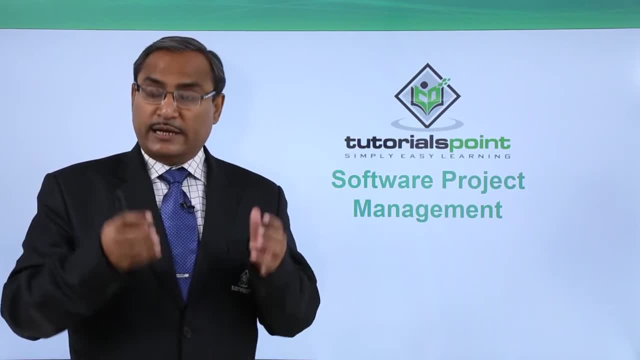 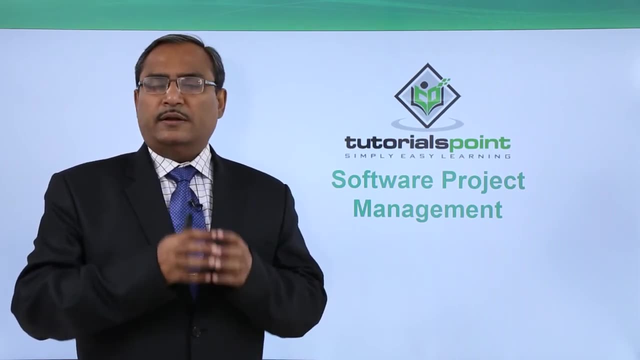 software architecture may differ, the requirements are different, The user interfaces are different, The functional and non-functional requirements are different. So each and every software is software development process is a project, Because at the end we are going to have a unique service. 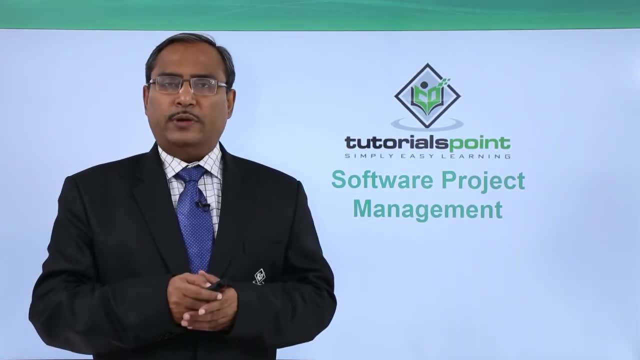 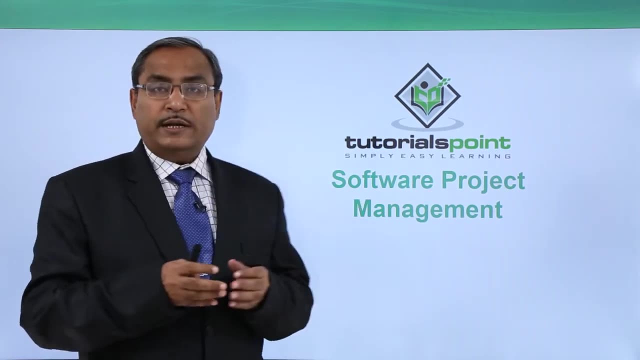 or product or result. In case of software development, we are going to get a unique product. So in this way, let us suppose I am going to give you the lecture on the software project management, If I, if you ask me to take this particular class. 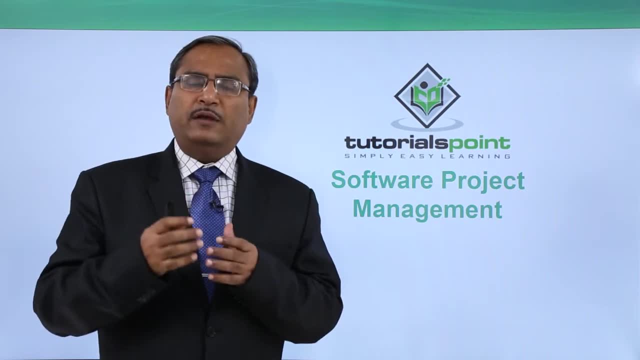 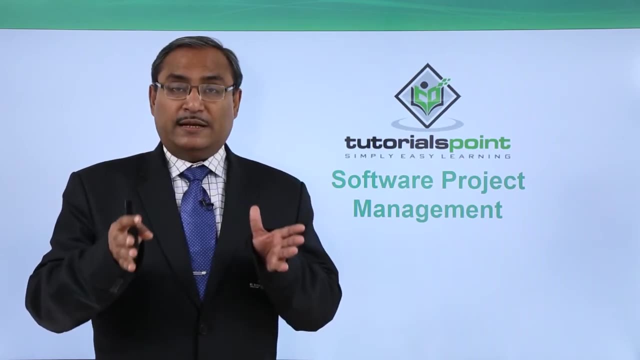 so say, for multiple number of times, Each and every time. I might be giving different sorts of examples, different discussion. I might be doing So. obviously, this class is this class. Whatever I am taking on this particular software project management, well, there, each and every time. 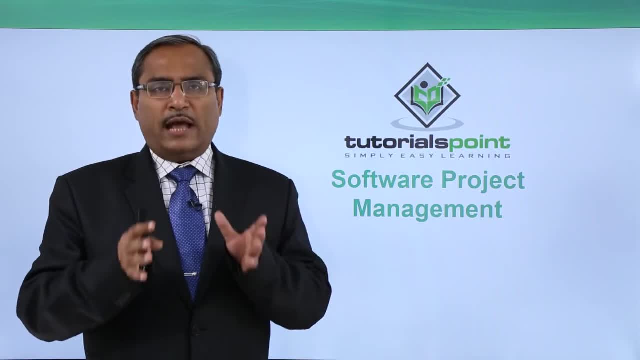 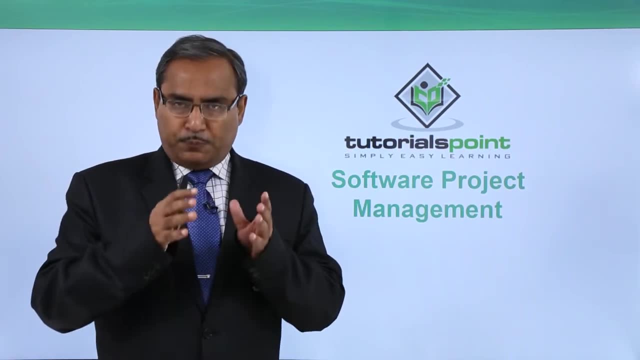 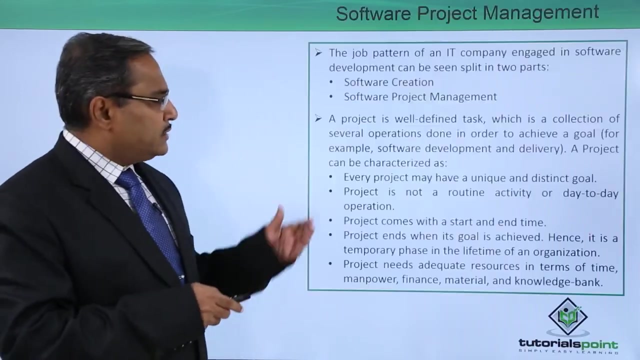 I shall give you unique service, So 1 as a project. so a project will be a temporary endeavor. that means it will have a certain start date and end date and the project should be ending up and landing up with one unique service, product or result. so now let us consider the software project management, so the job pattern of an IT. 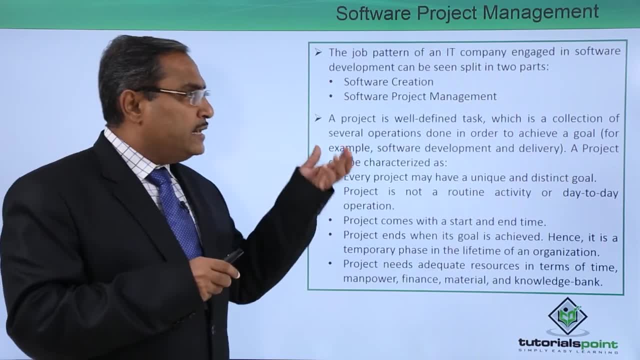 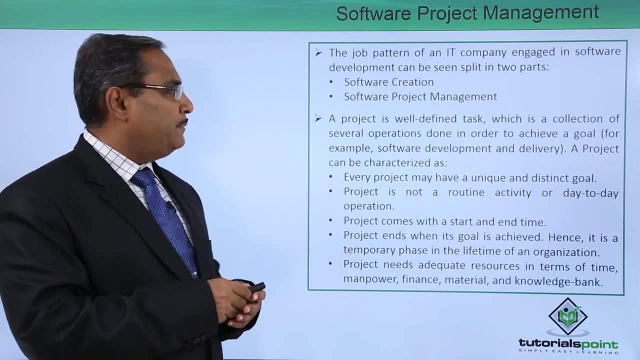 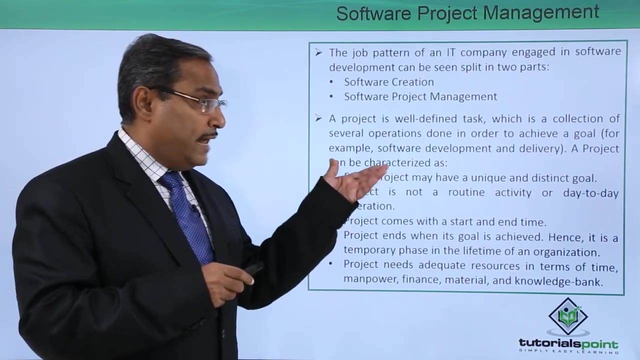 company engaged in software development can be seen split it into two parts. so what are the parts? one is a software creation and the one is a software project management. a project is well defined task which is a collection of several operations done in order to achieve a goal for 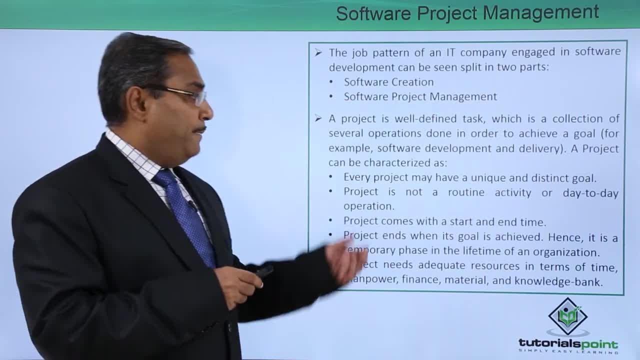 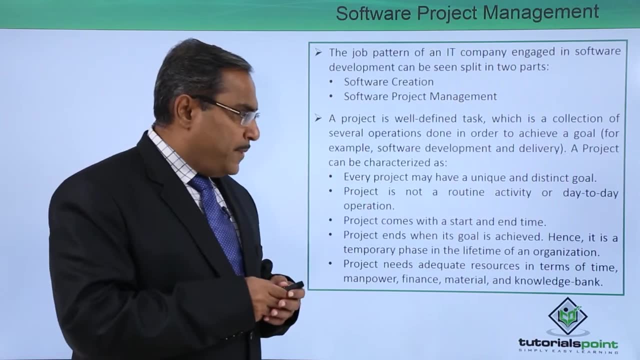 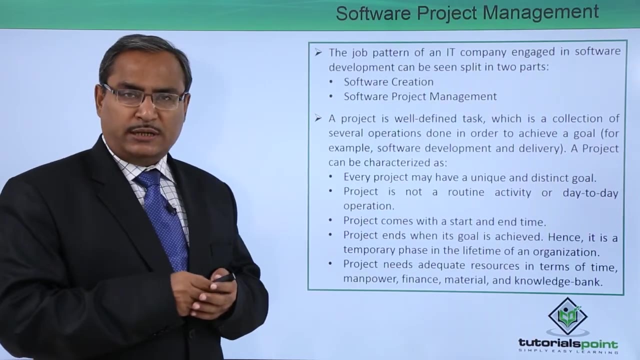 an example, the software development and the delivery. a project can have the can have the following characteristics, or can be characterized as: every project may have a unique and distinct goal. project is not a routine activity or day-to-day operation. you, if it is so, that means it is a production, it is not a project, and project comes with a start and